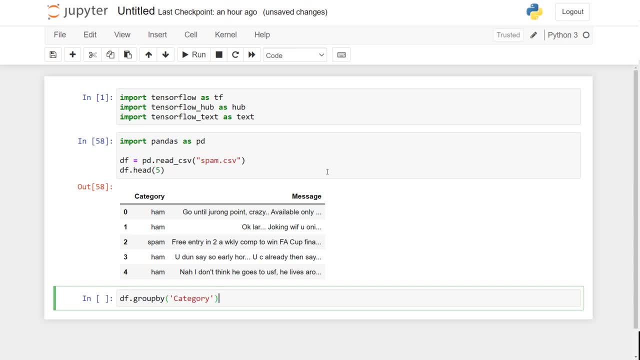 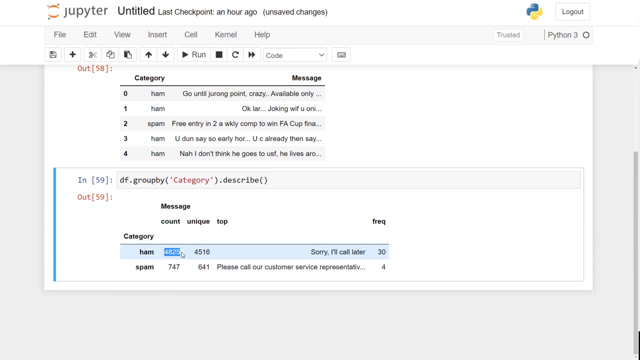 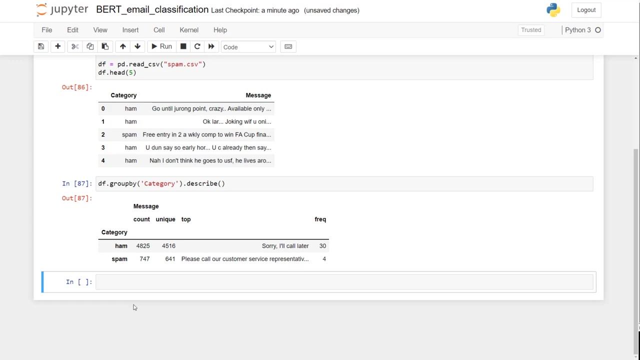 df group by, let's say, category. So here I have 4825 ham emails and 747 spam emails. You can clearly see there is some imbalance in our data set. The question is: how do you take care of imbalance in your data set? Go to YouTube, search for code basics, imbalance data set and you 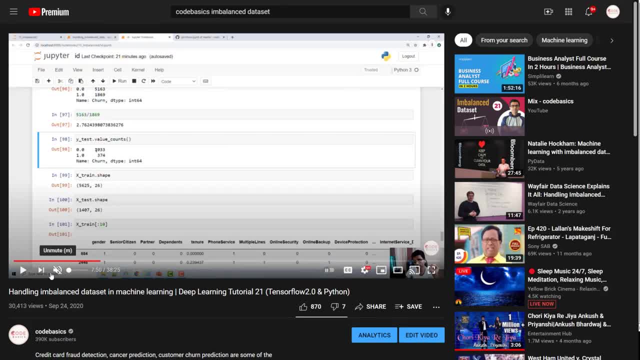 will find my video where I have outlined three different techniques for handling imbalanced data. There is a notebook. I think you should watch the video so you get an idea. I'm going to use a technique called. I'm going to use a technique called. 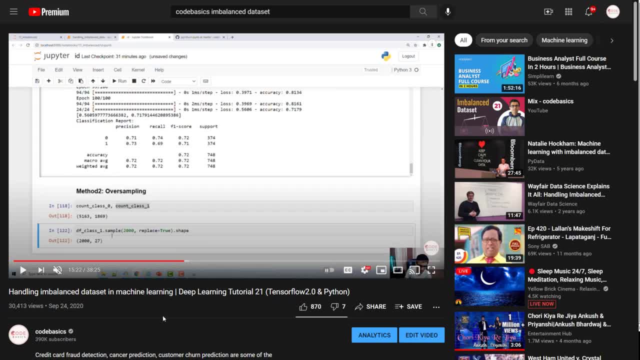 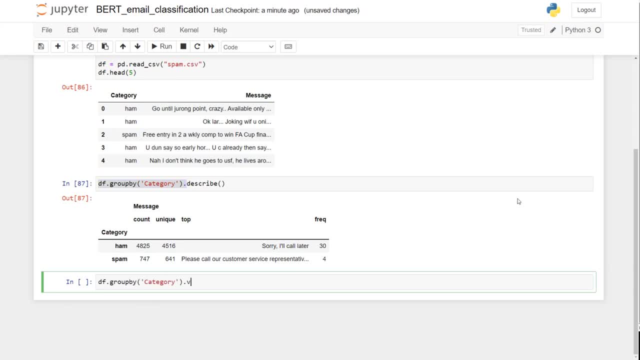 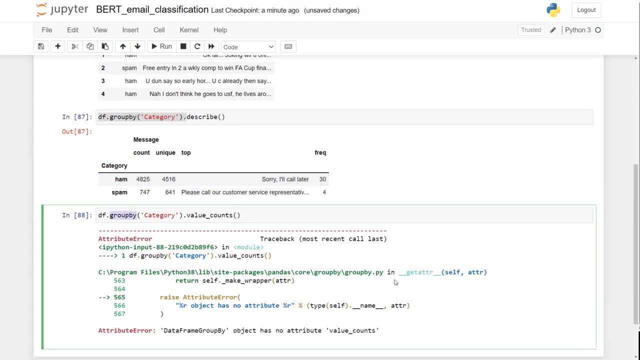 I'm going to use a technique called down sampling and what that means is it's pretty simple actually Here, if you look at the value down sampling and what that means is it's pretty simple actually Here, if you look at the value count, value counts actually. I should be doing this. 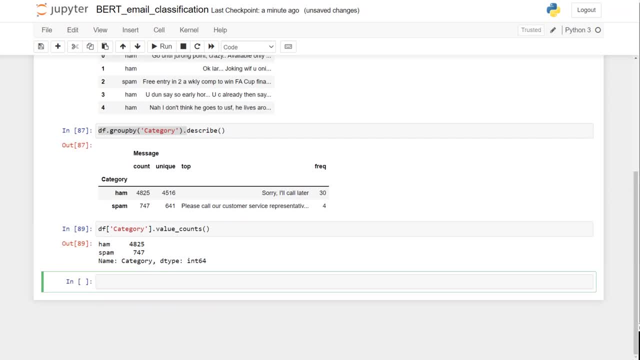 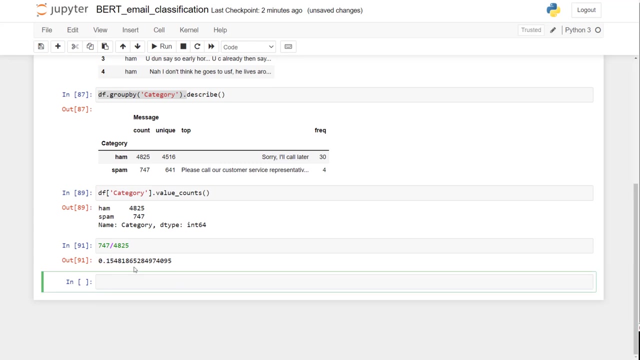 And if you check the percentage distribution, you will see that. actually, okay, you see that 15% are spam emails and 85% are ham emails, so there is definitely an imbalance. so downsampling technique: what it says is: from 4825 ham emails, just pick any random 747 samples. 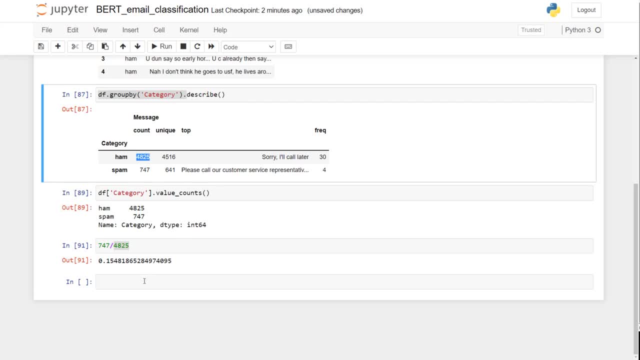 discard a rest of them that way, then you have equal number of spam and ham email. now, obviously, when you're discarding rest of the samples, you are losing your training data, which in certain cases might not be good. but for our tutorial, just to keep things simple, I will go with that approach. there are 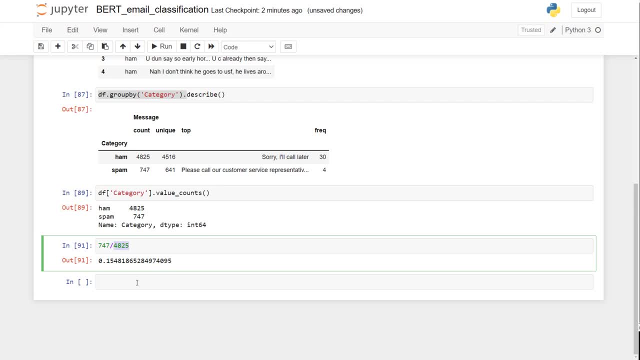 other approaches, such as smote oversampling- basically oversampling the minority class, etc. so you can watch the other video and you can try some other approaches, but I'll just go with a simple approach here. I will create a new data frame called VF- spam, where I would say D, F category is equal to spam. okay, and let's print the. 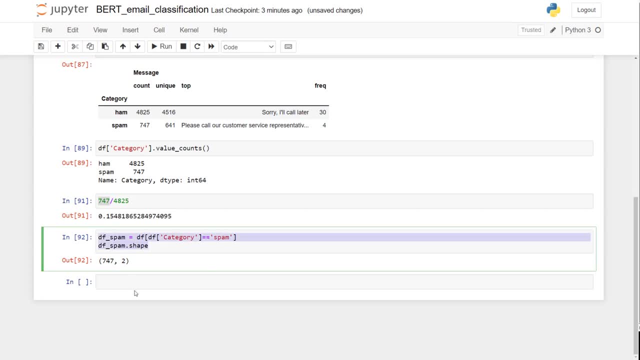 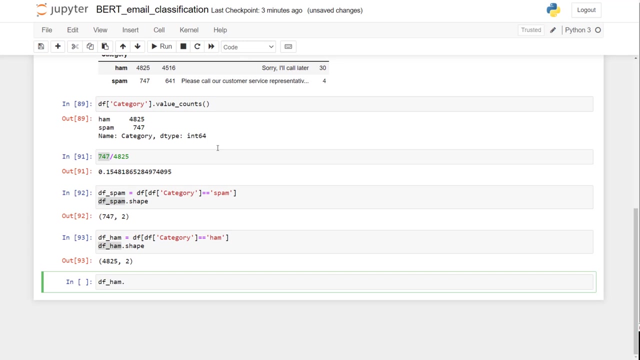 shape. obviously the shape. this is what you would have expected, and I will do the same things. ham. so I'm creating a separate data frame for ham and spam email. this data frame has only spam emails. this data frame has only ham emails. and now I need to sample this ham data frame, and the way you do that is by doing sample. so if 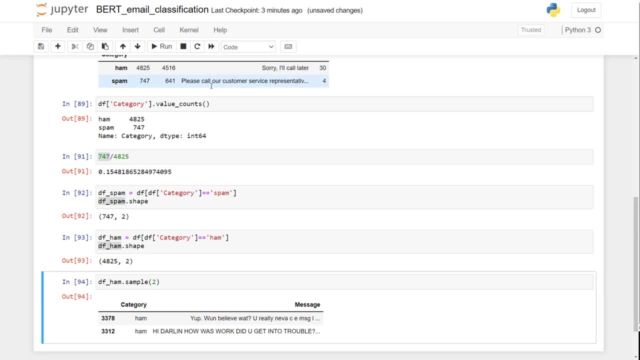 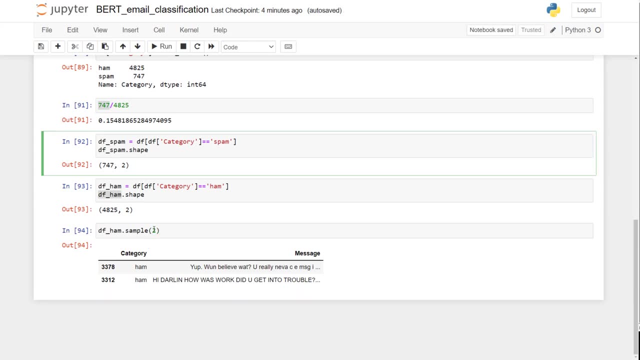 I do like, say, sample 2, it will only return me two samples. I want to sample 747 records, and the way you do that is, of course, you can type in 747, but in order to keep the code in a good condition, I will just do this, so shape. 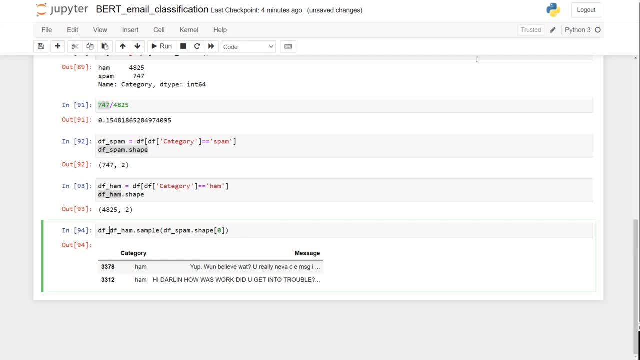 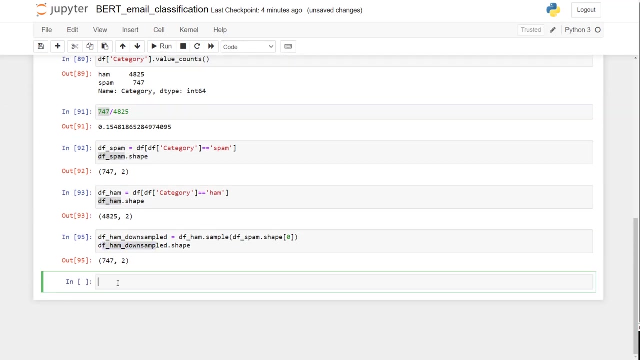 0 will return 747 and that I will call ham down sample and I will just print the shape just to make sure. see, both are now 747, this is 747, this is so for 747. I would now concatenate both of these together to form my DF balanced. yeah, so I will call it DF balance. data frame is equal to. 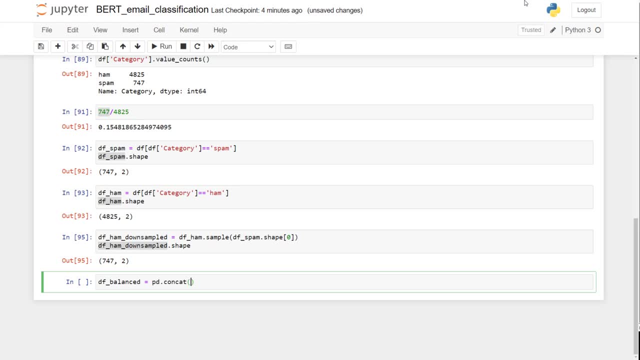 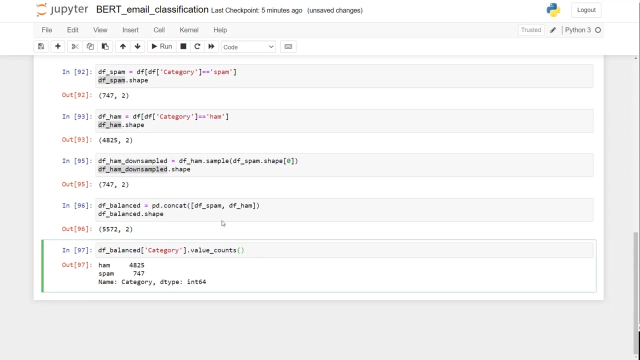 pandas PD dot concat. so concat is the function, and in here you can supply the data frame, and then you can supply the data frame and then you can supply both your spam and ham spam and ham data frame. I think that should work. and now, when I do value count for this guy, the value count is still approximately. 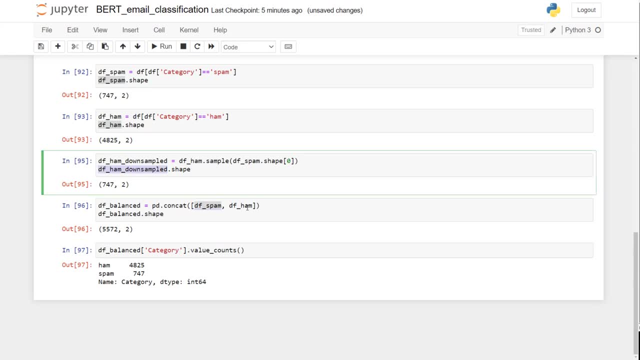 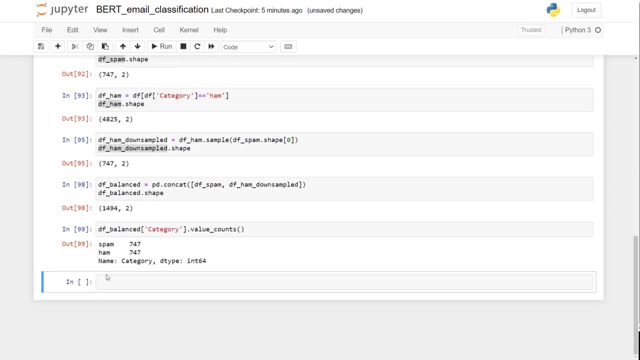 foron. let's see. oh yeah, I think I made a mistake here. I should have done this. okay, all right, now I have equal number of spam and ham emails. I discarded rest of the sample. I just picked 747 samples from for ham category. discarded rest of. 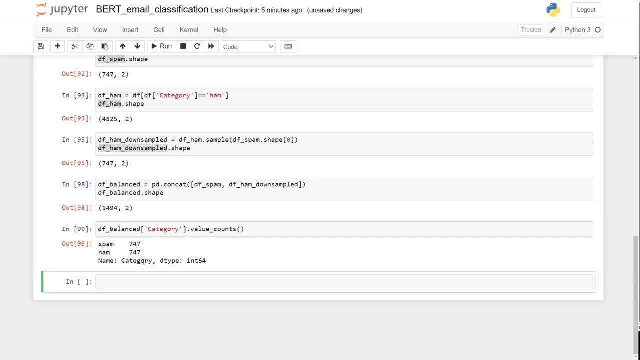 it again. that might not be considered good because you're losing valuable training data set, but the goal of this tutorial is to to explain you. but- and that's why I'm just keeping the thing simple- for other approaches, like smooth, etc. you can watch my other video and in the balanced data. 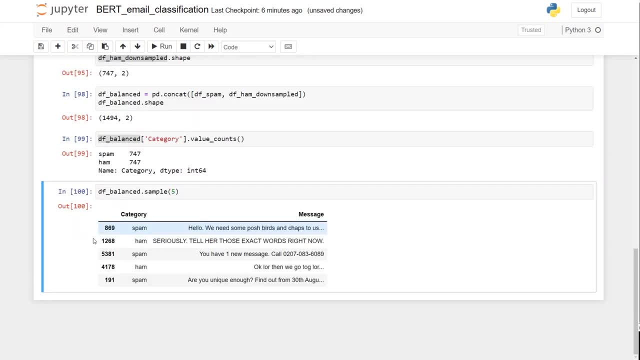 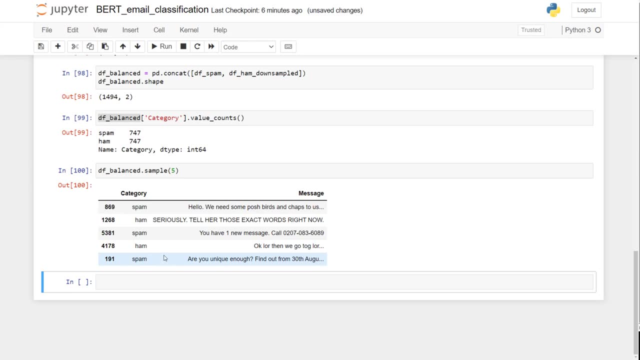 frame. you know, if you want to print few samples, you can print just to make sure things are good. now I would create a new column called spam, because here it's a text column. I want to create a binary column called spam. you know boolean like 1 or 0, that kind of thing, and you know how to create a new column when you do. 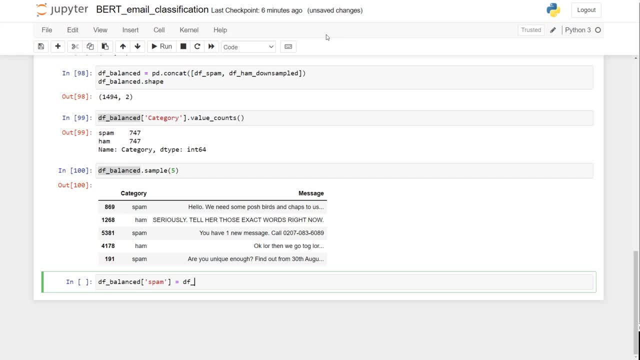 this, it will create a new column. and the way you create a new column is you go through the existing data frame, the category column, and you use the function apply. so if you've seen my pandas videos you will get an understanding that on category column we are applying some transformation and that transformation here you can define. 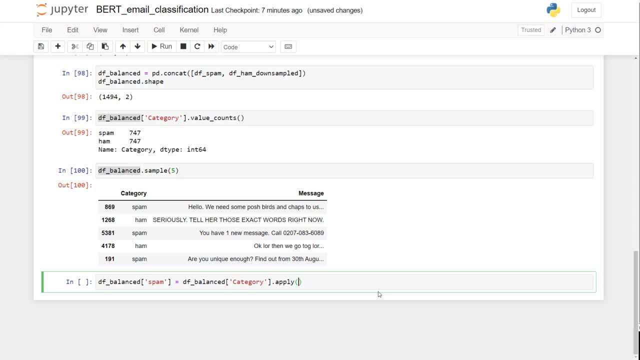 any Python function, okay. but here, since this is a simple function, I will just use lambda. lambda is a quick way of writing a function and I will say: okay, if, if my X, what is X? each of the values in this column category. let's say if X is. 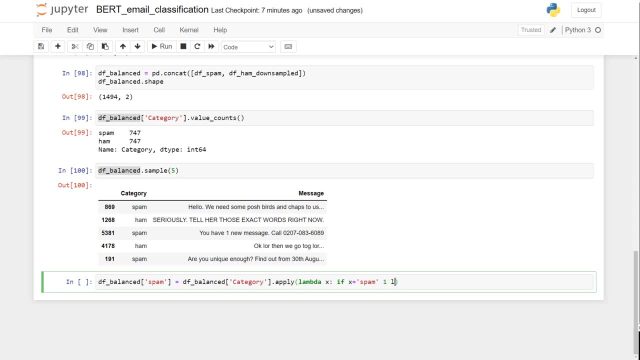 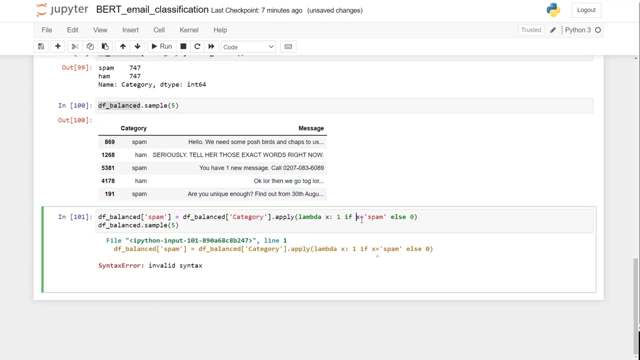 is spam, then the value is 1, else 0. this is the correct syntax. you're saying 1 if X is spam, otherwise 0. I would again sample it, just to make sure you know my new column is created properly. so let's go ahead and multiply whatever you write. so what you're doing here is: 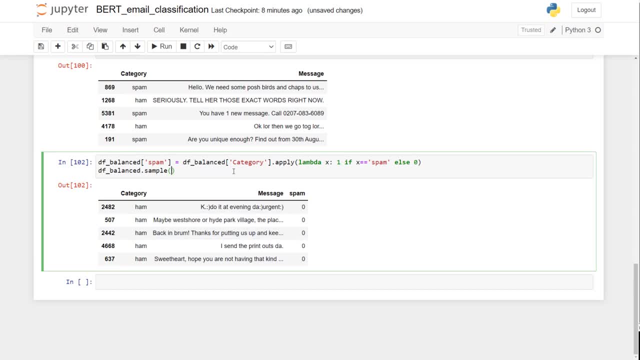 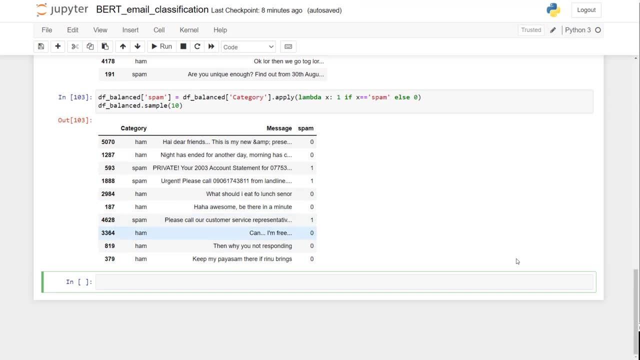 taking a part two of that, part two of the mean, you'll use the value and then multiply by 2 and 2. what do you mean by multiple number? okay, so you get that one more two, two times. so we can do it that way too. meanwhile, let's see if we did it right. so next time we'll be adding a new. 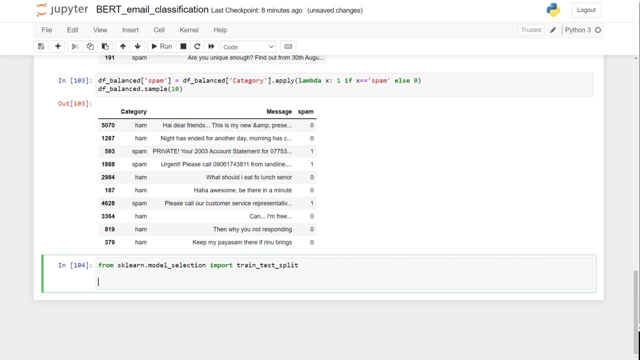 build query. we'll be adding a newFrame and a a copy of that. whether you have mentally tested it or maybe you've gotten an early version of the code, can we combine those two things into one form? you will use stratify so that in your train and test sample, the distribution of the categories 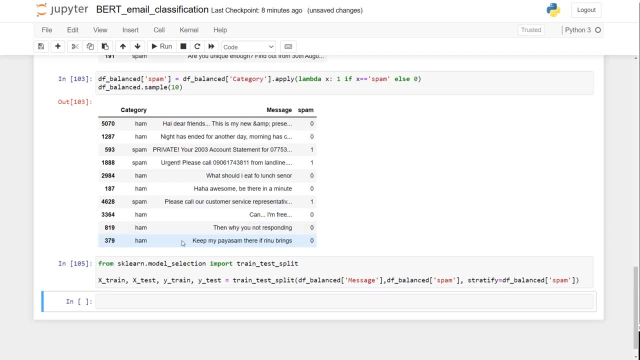 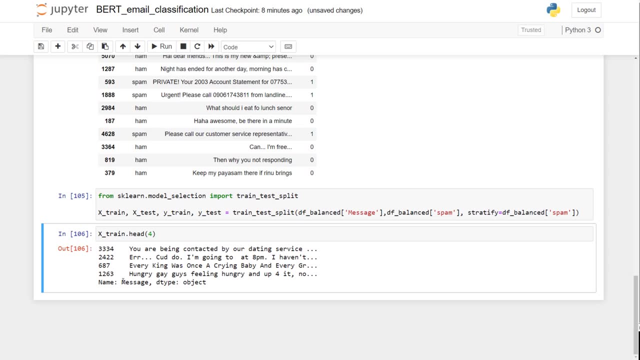 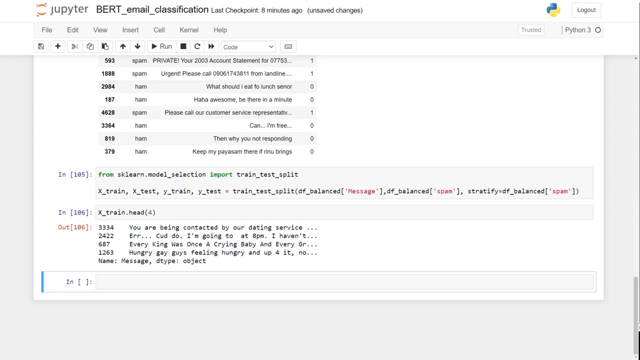 is equal. all right, my x-train etc is ready. I will just print the head of x-train just to make sure. great now comes. but the most important part, all right. so, but in our previous video we have seen how can you create the preprocess and encoder model, encoder object, and I'm just going. 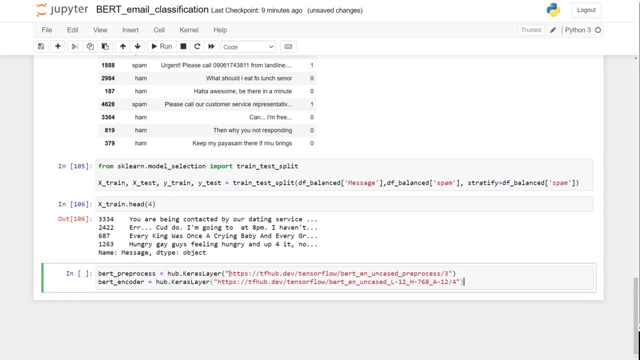 to copy paste, because we have covered this in our previous video. just to summarize, on tensorflow hub website, these trained models are already available, so you're just using this URL to download it and then you can use it to create the code, and then you can use it to create the code. 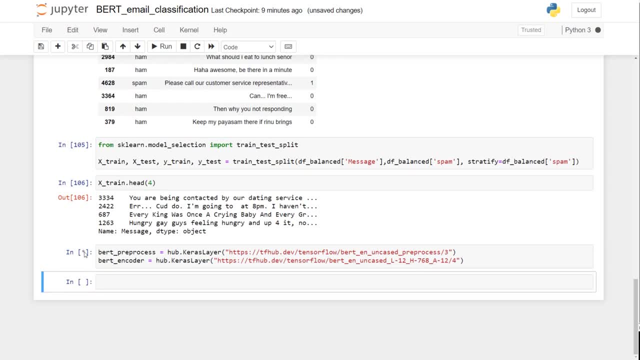 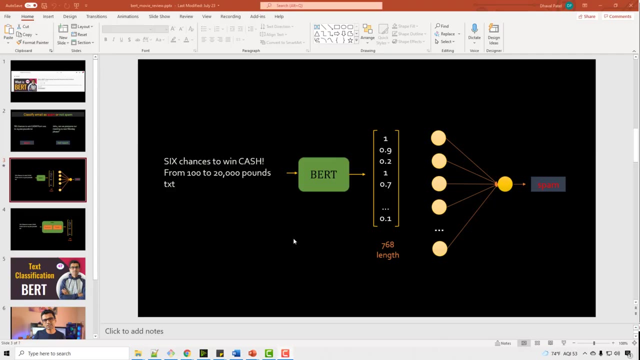 load those train models and you will realize that when you execute this, you will see star for a few seconds or minutes based on your speed, because it is downloading the train model locally on your computer. now, as you have seen in our presentation that my goal is to supply sentence to BERT model and create this length vector, let's write a simple Python. 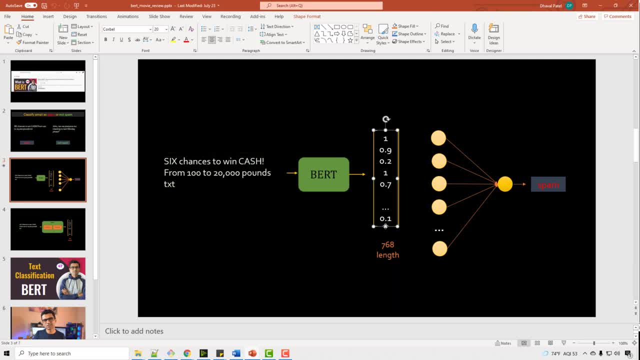 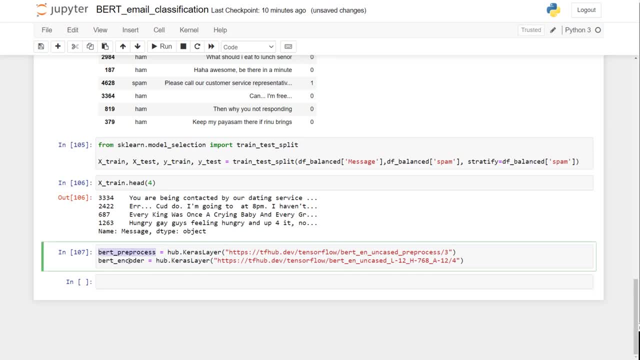 script, and then we will see how to do that in our next video function that takes this sentence as an input and returns this vector as an output. meanwhile, this download got completed, so my BERT preprocess and encoder is ready. I want to write a function, you know, something like this: 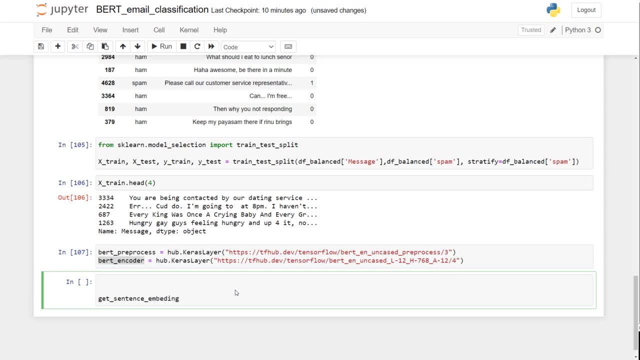 when I say get sentence embedding and when I supply a sentence like this, it should just return me 768 length vector. now to make this function more versatile, we can take an array, okay, so we can supply basically multiple statements, so that will return, you know, multiple 768 vectors. so here: 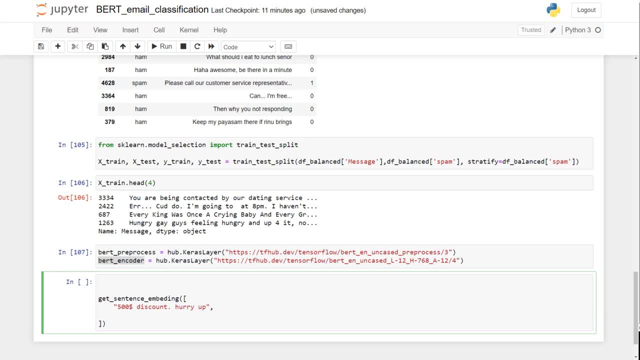 um, i'm just putting any random statements. you know you can put whatever you want, and the goal is to write this particular function. now, if you have seen my previous video, i would ask you to write this yourself, without relying on me. a good student would pause this video and write the function themselves. 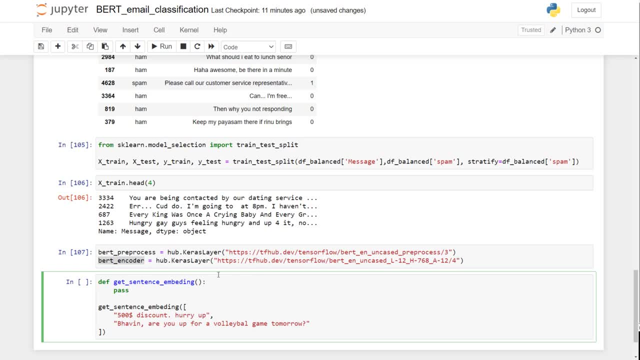 all right, considering that you have attempted, now I will write this function. it's pretty simple actually. you are getting sentences as an input and you call preprocess first, correct. you call preprocess on your sentences obviously and you get the. actually there is a spelling mistake. so you call preprocess on sentences. you get. 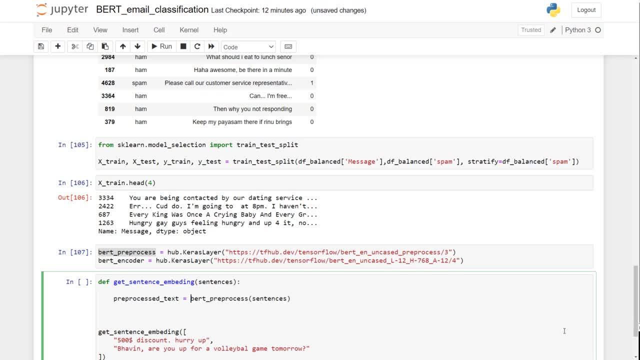 preprocess text as an output and that you supply into bot encoder. the code is so simple, friends, it's just like a function pointer. you know it's a simple function. so you are doing preprocessing first and then you are doing the actual encoder. now the encoder will return a dictionary, but from that dictionary you 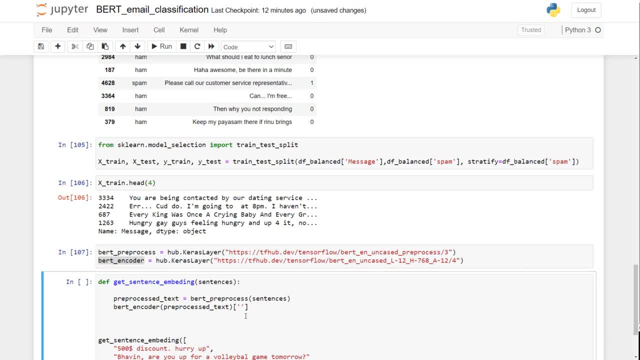 need to choose a pooled output. we have talked about that in our previous video. so, again, if you have not seen previous video, you will have some difficulty understanding this particular video. that's why watching previous video is very much essential. I'm just going to return this, by the way, and that would be. 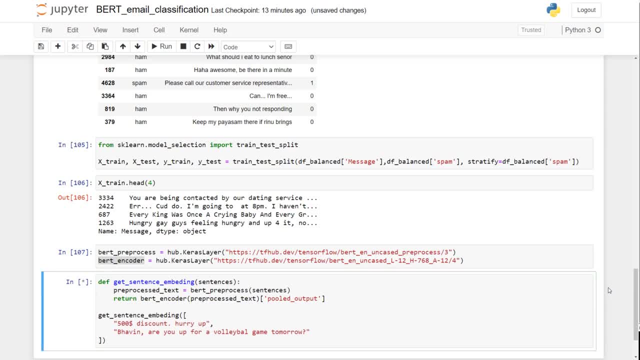 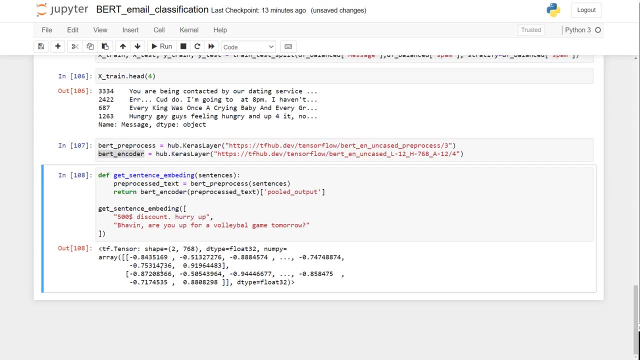 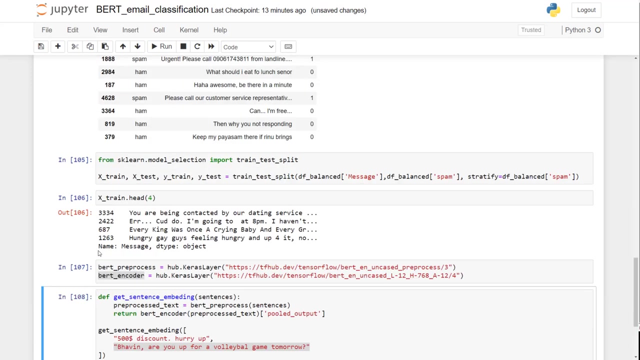 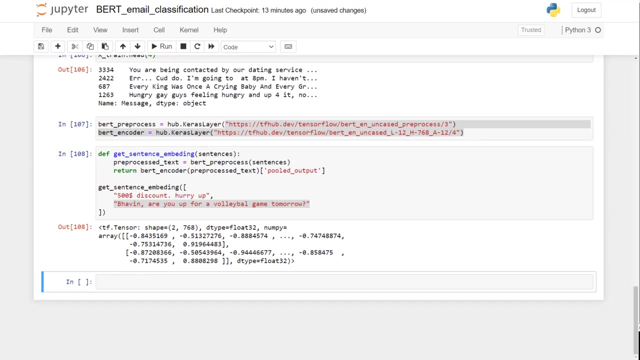 my sentence encoding and when you run it you can see it's returning a tensor of shape to 760. so this particular tensor is my sentence and encoding for the first sentence. for the second sentence, here is my encoding and this encodings are returned by pre trained BERT model which I have downloaded from TF hub website and 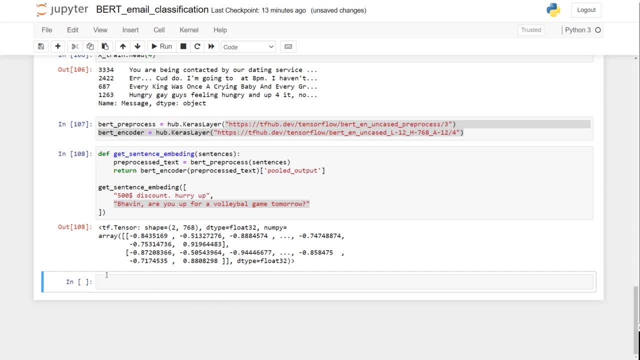 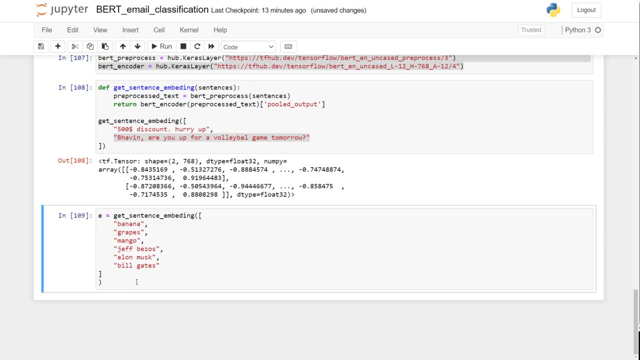 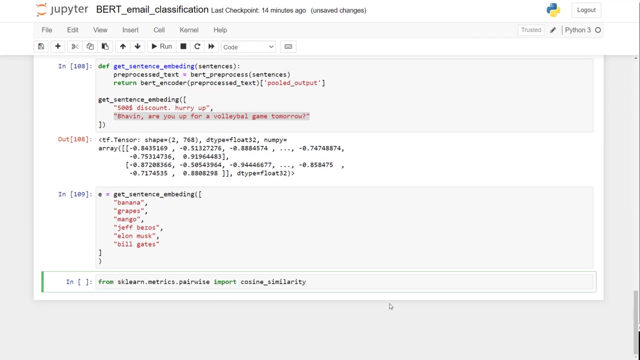 great, now let me call sentence encoding for some simple words you know, like banana grapes, mangoes and so on. I want to see what this really means. what, what, what is the benefit of having this BERT encoding? so I will try cosine similarity. cosine similarity is a way to measure how, how, how similar two vectors. 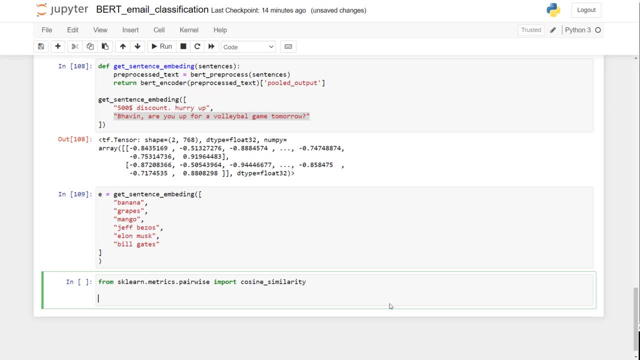 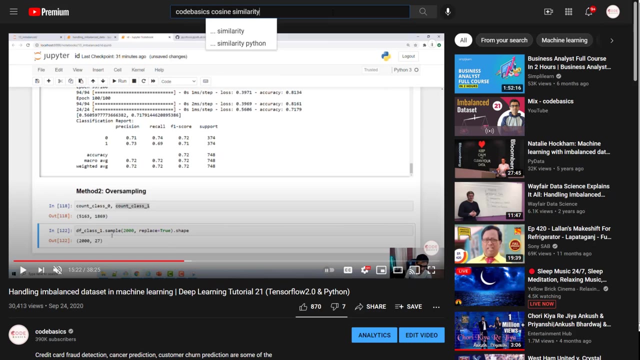 are. if two vectors are pointing in the same direction, then that means the cosine similarity is will be close to one. now if you don't know about cosine similarity, you can do core basics cosine similarity. you'll find a very simple video. I try to make it as simple as possible. 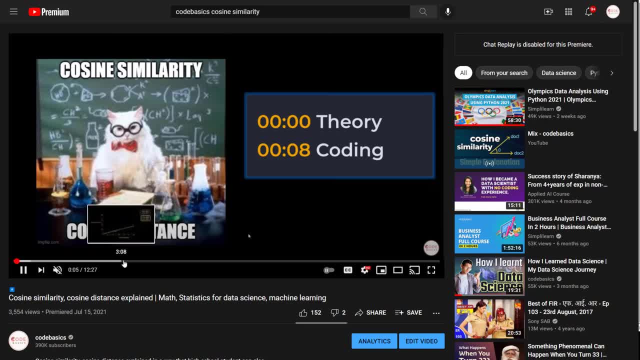 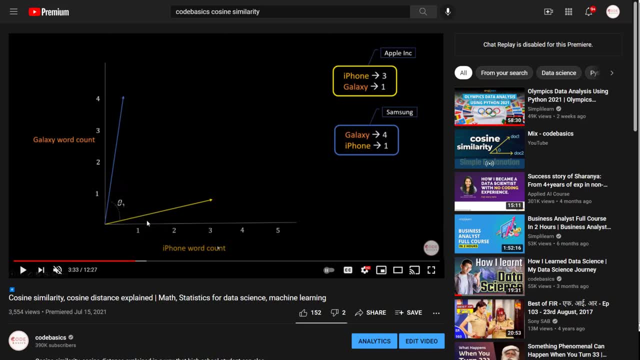 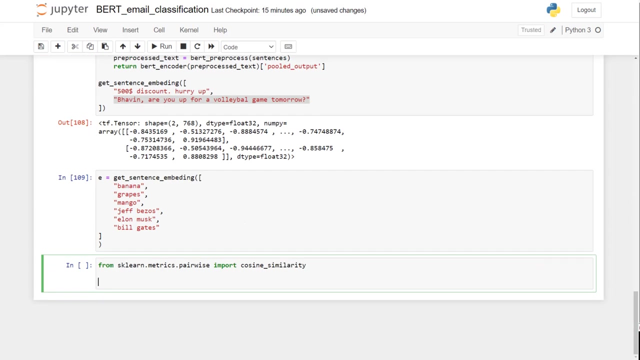 videos which even a high school student can understand it easily. and here I have explained that if your vectors like this, where the angle is more, then you know the similarity is less, but if you have vectors where the angle is less, then they're more similar. okay, so that that's pretty much about it. so, cosine. 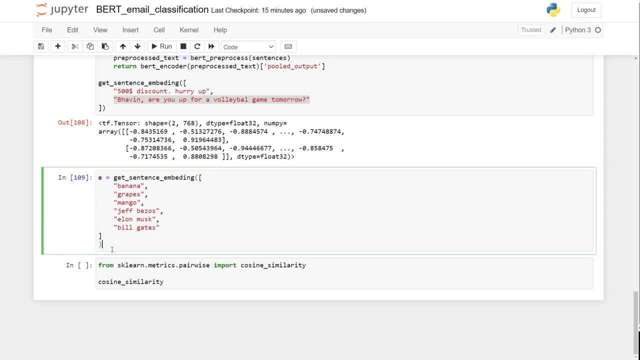 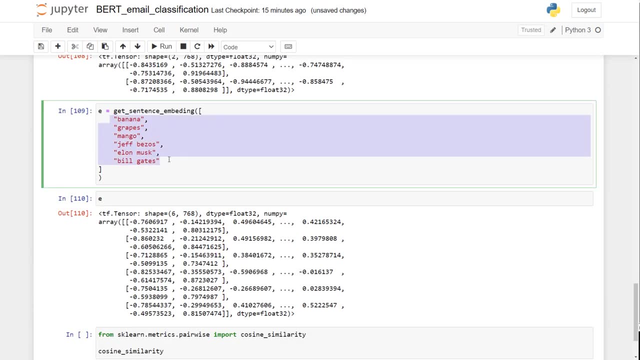 similarity. I will call now. so this E, by the way, let me print: E is the embedding of all these words: banana, grapes, mangoes and so on. I got six embedding. each embedding is a vector of size 768. you would now think that the first three vectors would be similar. their cosine similarity, they. 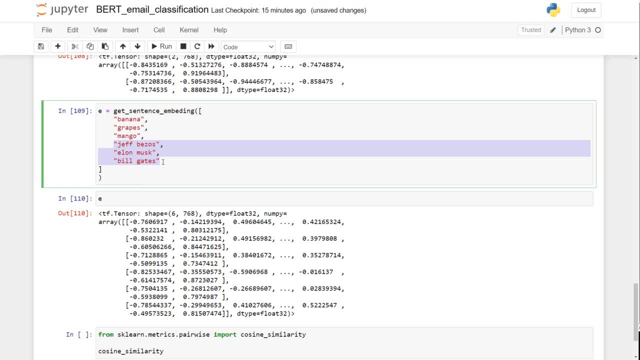 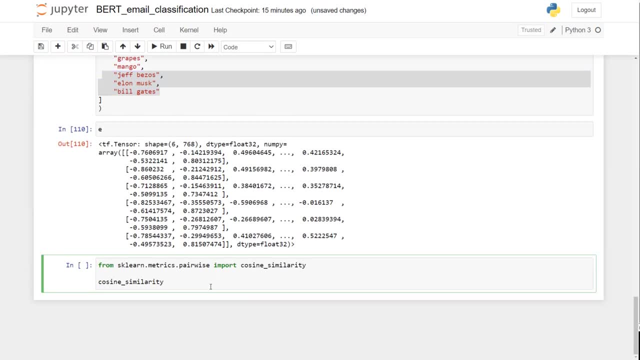 would be similar in terms, of course, higher similarity, and these three would be similar because these three are fruits. these three are not fruits. obviously you know that they are entrepreneurs. here I would say: embedding 0 and embedding 1. now this expects two dimensional list. that's why I'm just putting two-dimensional list here, see, 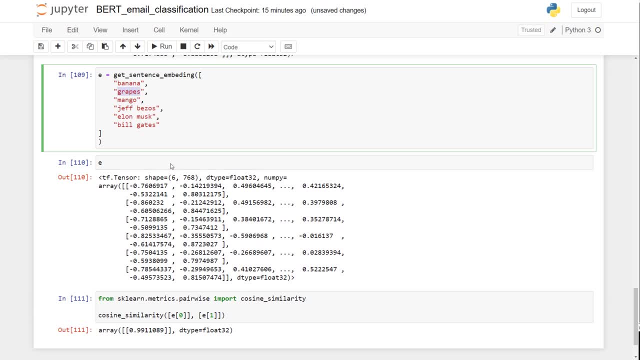 banana and grapes are very similar, but if you do banana and Jeff Bezos, let's do that. so, by the way, 0.99 close. if values close to 1, it's similar. 3 is not that similar. I know it's point 84, so it's the similarity. is not like it will capture. 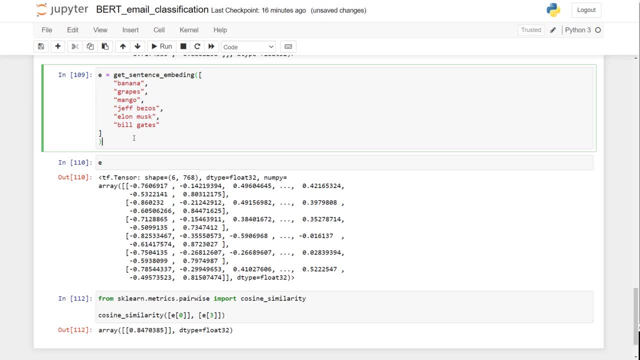 the. you need to understand how these embeddings are calculated. they are calculated based on- based on the training that they did on Wikipedia and Google books, where based on the context, so based on a context. as such, profit and loss will also be similar. so you need to understand that. okay, it's not. it's not a. 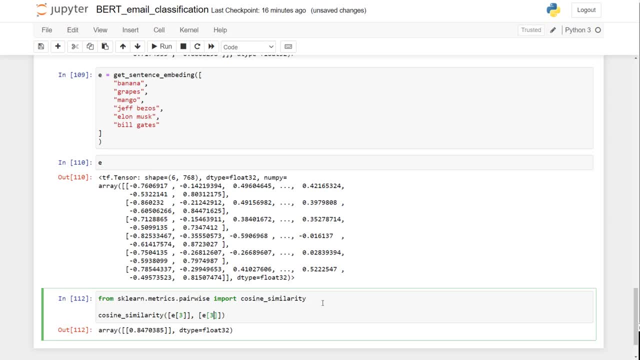 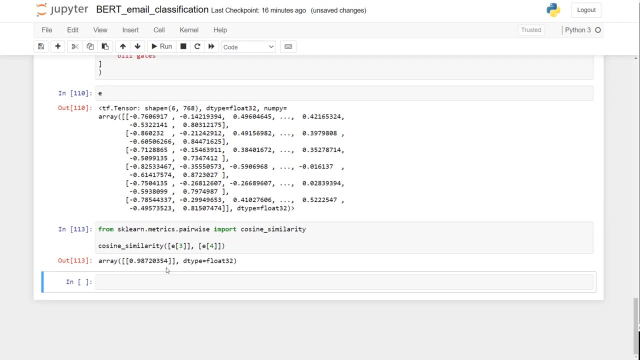 silver bullet here, but if you do like 3 and 4, 3 is Jeff Bezos, 4 is Elon Musk. see 98%, because when the train board model on all the Wikipedia text, the context in which Jeff Bezos and Elon Musk appear would be similar. 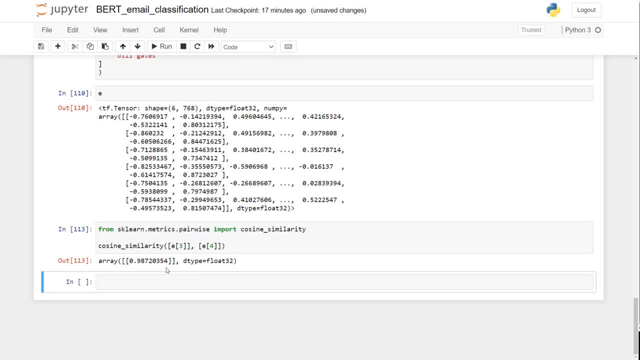 when they will be talking about Jeff Bezos, you will see words such as entrepreneur, rich, you know, like company name that plants, and so on. so that's why their Cosine similarity is similar. anyway, you can play with it. but let's get back to our main objective, which is to build a classification model. so now, 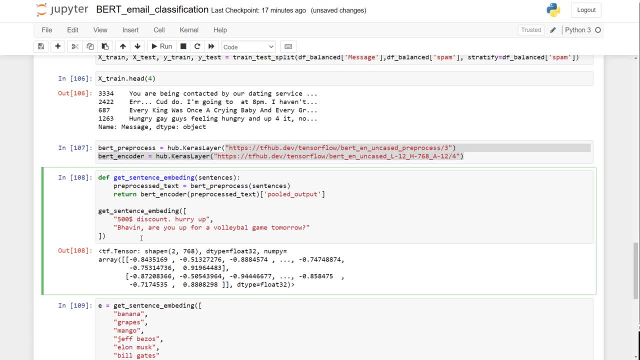 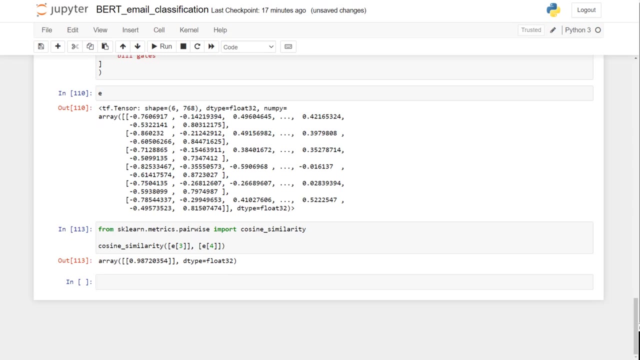 we have this function which is returning the sentence vector losing class backs to the class Pues. channels are calculated based on the presentation. but I mean we are not going to use this function. we will be using these, these two pre-processing and encoding functions, into our BERT layer. now I'm 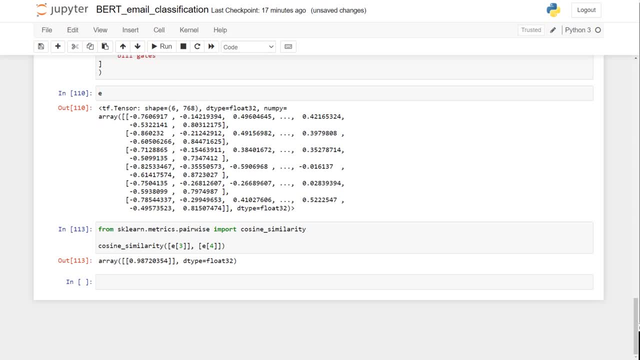 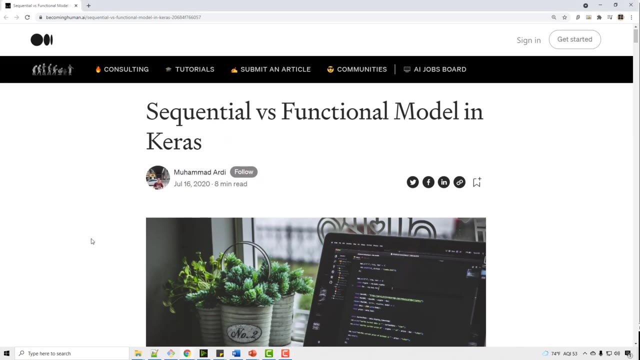 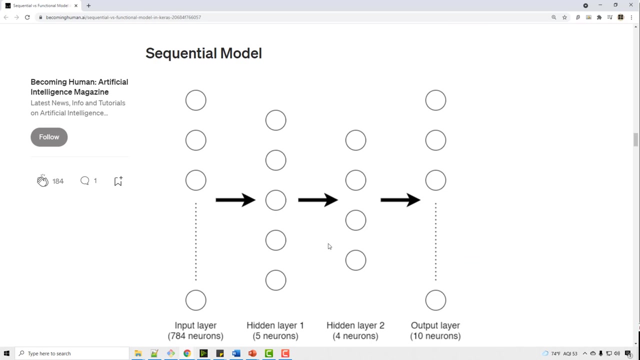 going to create a model. so there are two ways of creating the tensorflow model: one is sequential and one is functional. I would suggest you read this article of regarding sequential and functional model. in our video so far, we have created sequential models which are which looks something like this: there is 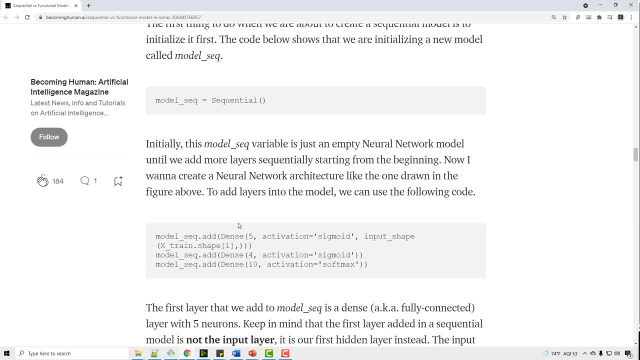 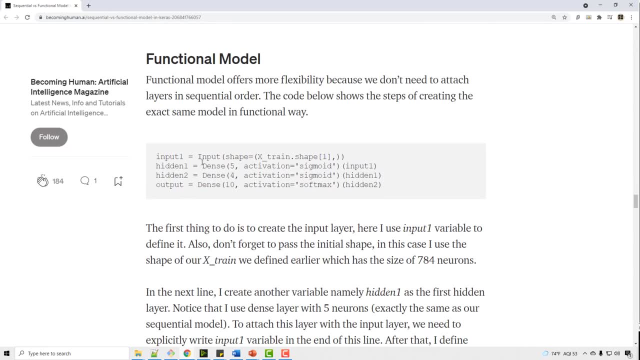 a sequence of layers and you know how to create sequential model, because that's what we have done so far. but functional model looks something like this: you create an input layer, then you create another layer and pass the first layer as if you are calling a function. see, as if you are calling a function, you're. 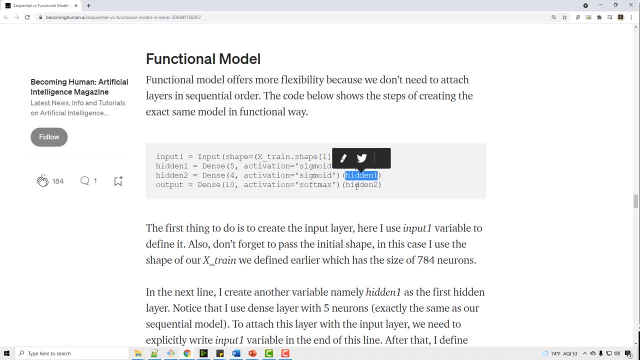 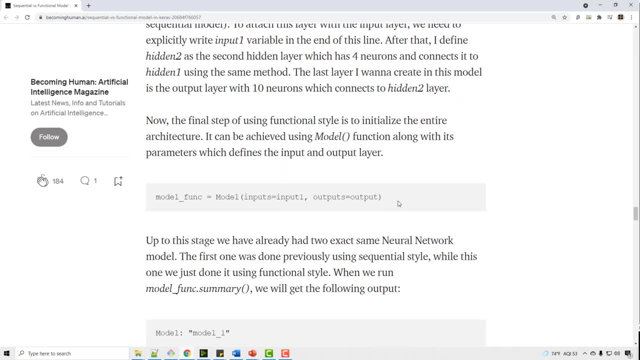 supplying this hidden layer as argument of this function and eventually we create a model. we say, okay, inputs is this and outputs is this, so output would be this and input is whatever you created. the benefit of this is that here you can you can have basically non, non sequential type of architecture where you can have 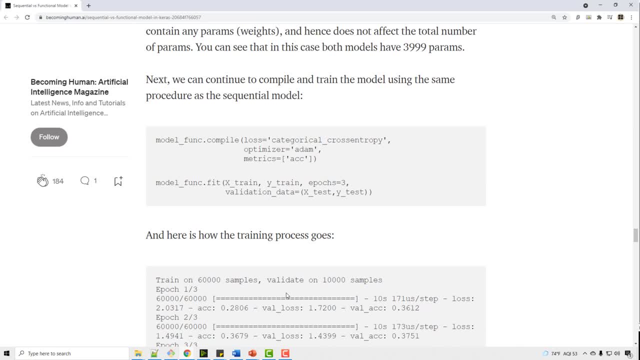 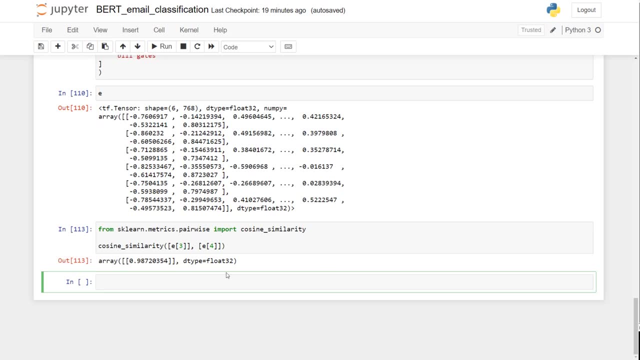 two inputs, two outputs. you know you can build complex models out of this, so we are going to use that approach. so let's first create our input layer. what is our input layer? so in an input layer I will say: shape is this. so I will let it. 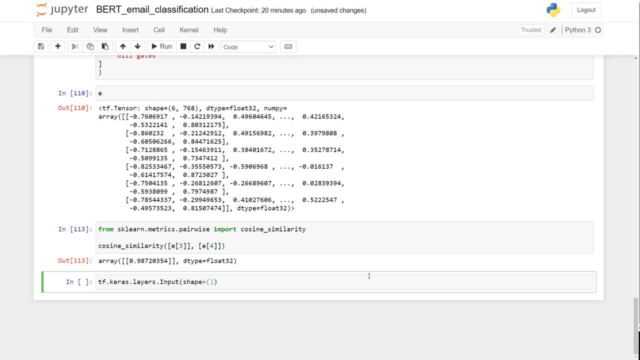 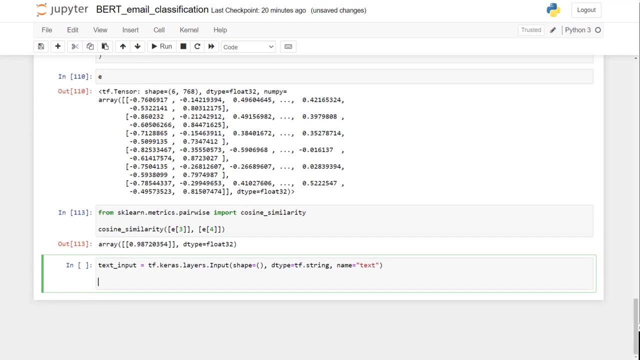 derive based on what encoding BERT is by passing, and then the data type would be tfstring and this is the name of the layer. you know you can give any, any layer and this is my input. again, if you read that article you'll get an idea. I created input layer. now that input 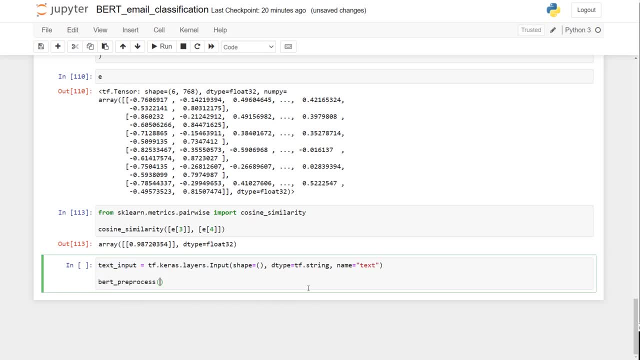 layer. I will pass it to BERT preprocess. what is BERT preprocess? we have seen it here. this is BERT preprocess and this is BERT encoder. so I'm passing that as a text input. what I get is a pre-processed text and that I 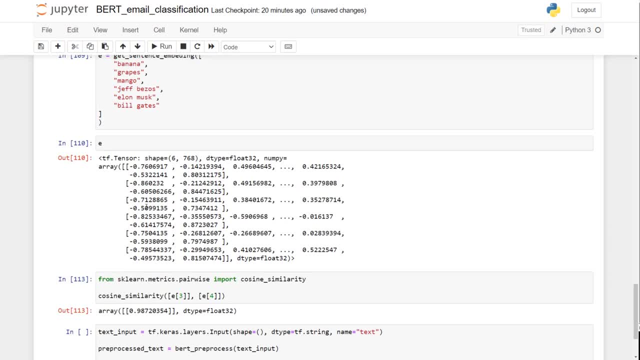 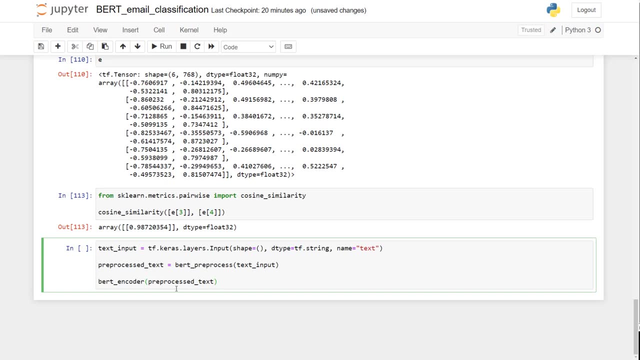 supplied to BERT encoder. okay, this is fairly straightforward and you get outputs as a result. so these are BERT layers, basically BERT layers. now I will create neural network layers. so in neural network I will create a dropout layer, because dropout helps with overfitting etc. so create a dropout layer and say, okay, maybe point one. 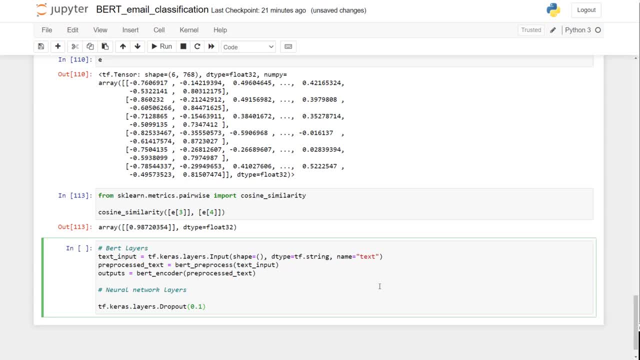 percent of neurons just dropped. I had made a separate video on dropout layer as well, so you need to go through that video. so this is dropout and since it is a functional style neural network, you call it as if this is a function and you need to supply. 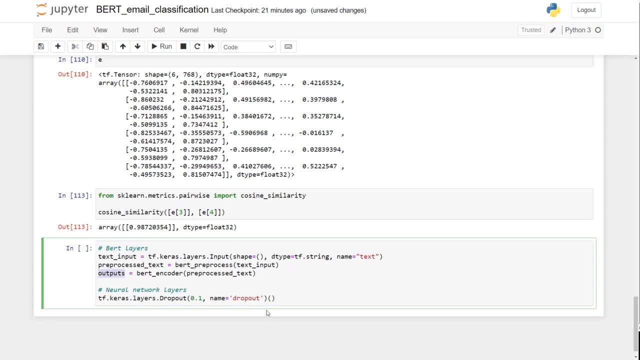 an input. now, what is the input? input is outputs pooled model, because, remember, the pooled, pooled output will have your bird encoding of 768 size vector. so that's my layer, i'll just call it l. and then second layer is dense, and this layer, by the way, has only one neuron, because one neuron is telling you: 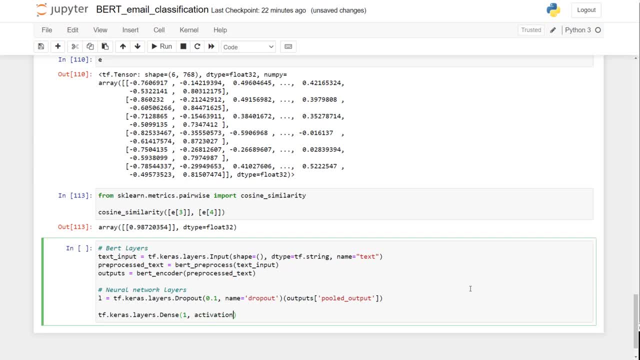 whether email is spam or not and activation is sigmoid, because sigmoid, you know, if it is more than 0.5, it's, it's spam, less than 0.5, not spam. just give any output, any name, and again, this is a functional style. so here in the function argument you will pass whatever you got from your previous layer. 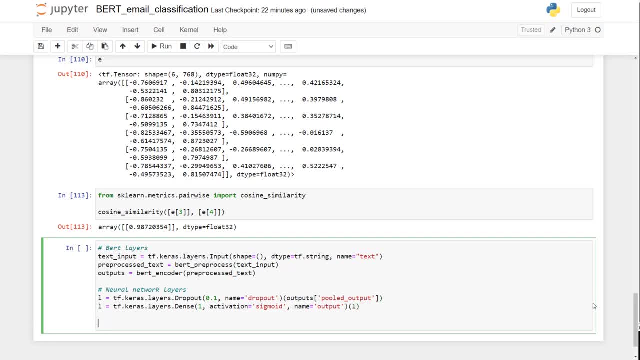 and i'll just call it the same variable. so now i got my neural neural network layers defined, i will construct a final model. now, construct a final model. how do you do that? well, do you bother, graham? word node string input in a 했 google. console- does it just rocketists- allows you that we can do seeking. if you work out that you will point selvain- until you have multiple output layer. multiple input layer- this architecture allows you that we can use sequence data rather than lectures. come if i have multiple outputly. so if you want to do multiple output you. can get it as an array and if you have multiple output, you want to get my output layer multiple things. this architecture allows you that. Suppose that we remove the linear expert and then do it automatically. code side. we have our certain columns which we don't want to melonds to. 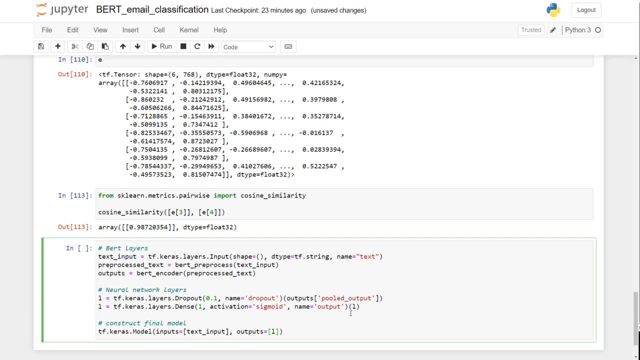 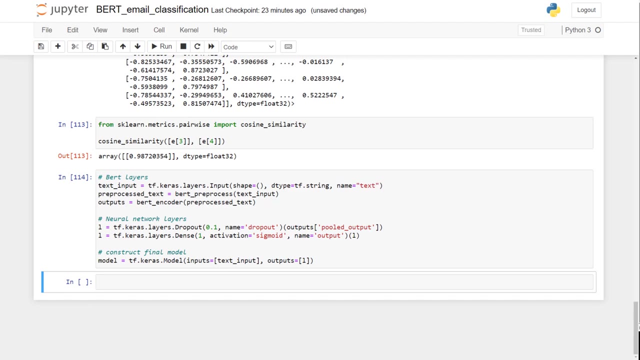 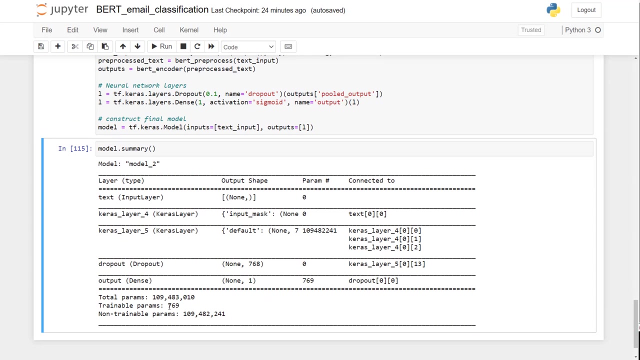 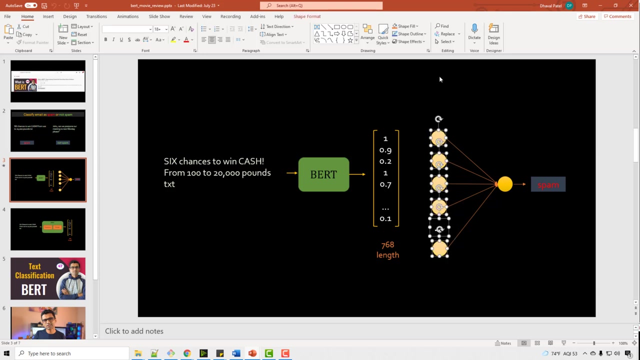 here as well, we are not using multiple input output, but this is just for a demonstration. so here I got my model and I will just control, enter. okay, just print a model summary to take a look. here you see, trainable parameters is 769 because 768 is my input. so if you look at our diagram here, so this, this layer, will be of size 768. so 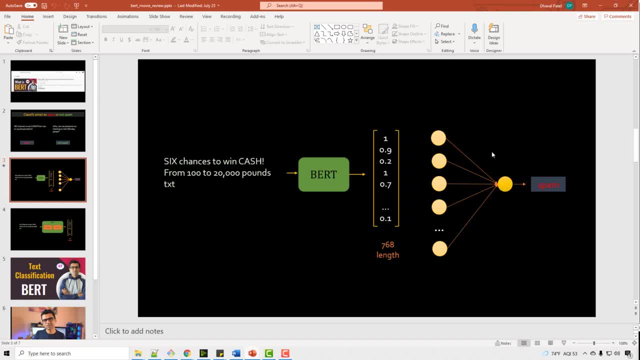 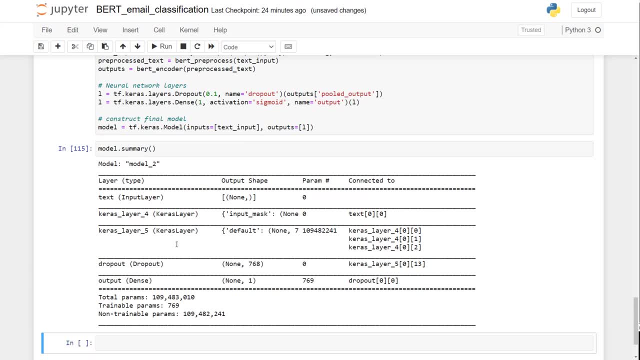 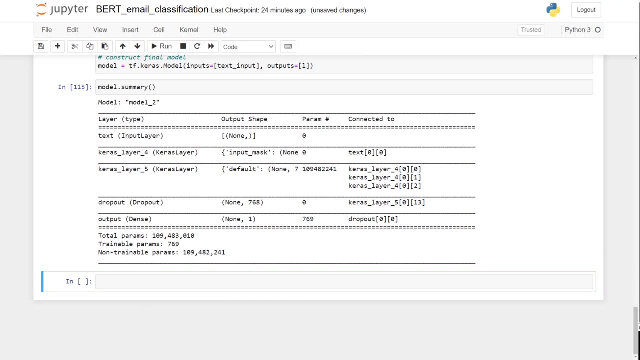 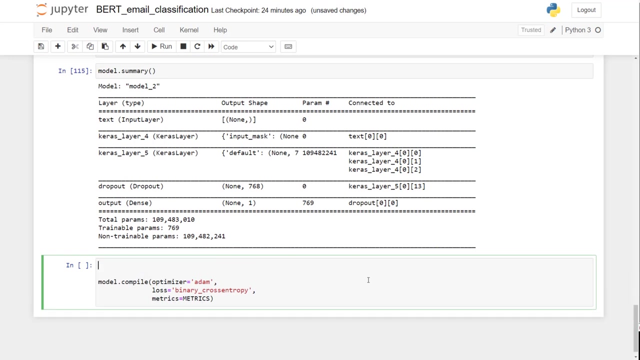 you need to train those parameters and one parameter for this. so 769 and remaining parameters are non trainable because they are coming from BERT and we don't need to worry about retraining them. okay, now comes model compile and we will pretty much use Adam as an optimizer. loss binary cross entropy. 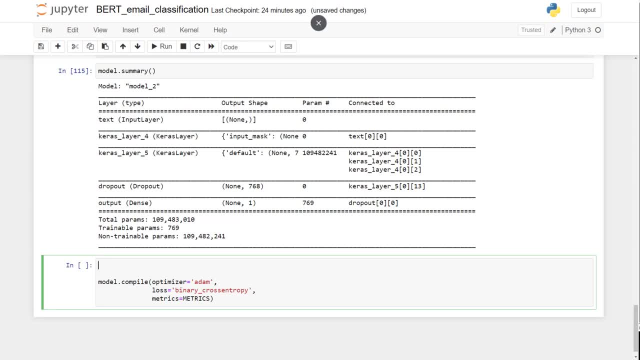 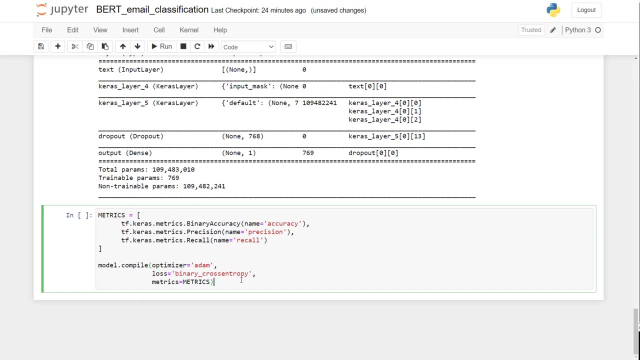 because our output is binary 1: 0 into the matrix. I will use a couple of them, including accuracy. I will use precision recall. by the way, when you supply matrix, it doesn't have impact on the actual training because the training is driven by loss function. but 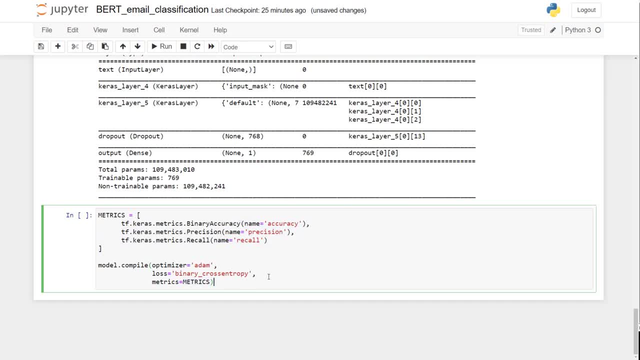 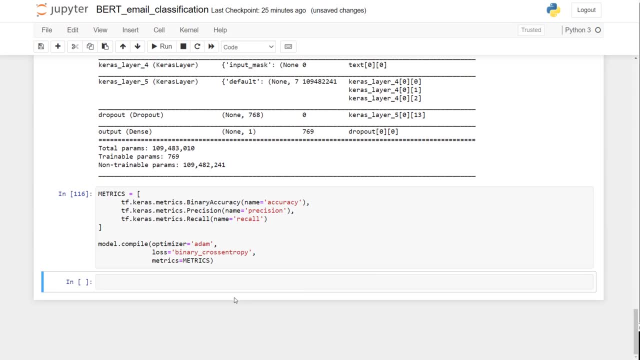 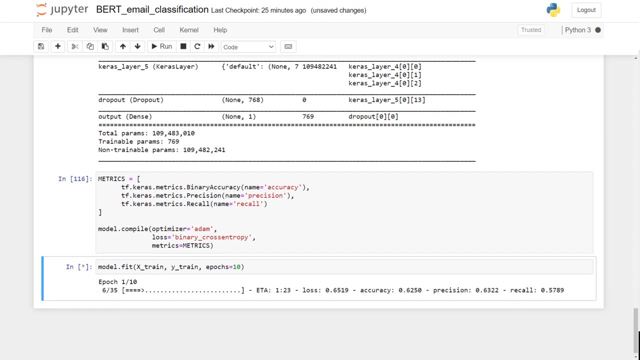 the matrix is just. you are just printing this number so you get an idea on how your training is working basically and you will do model of fit I. I would just go with tan Epochs. training is a little slow but you can see every iteration. it is printing loss accuracy. 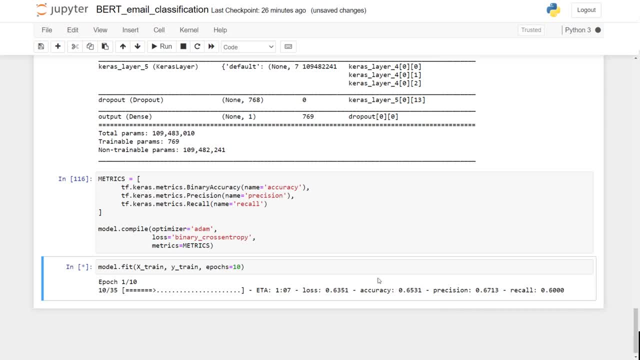 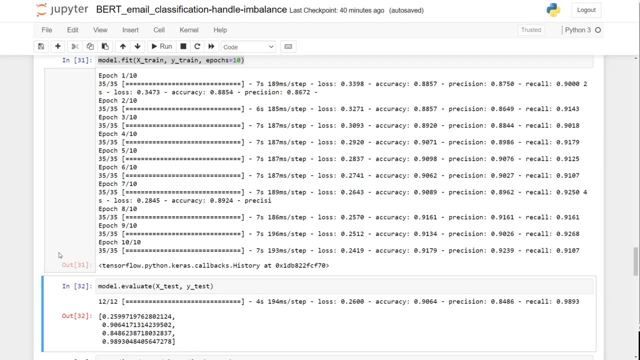 precision and recall. it is just printing those metrics. the actual training is driven by this loss function. it took some time but eventually my accuracy came out to be 91 percent. precision and recall is this much. now I made my data set balance so I can rely on accuracy. but in general, if you are training on imbalance data set, you should. 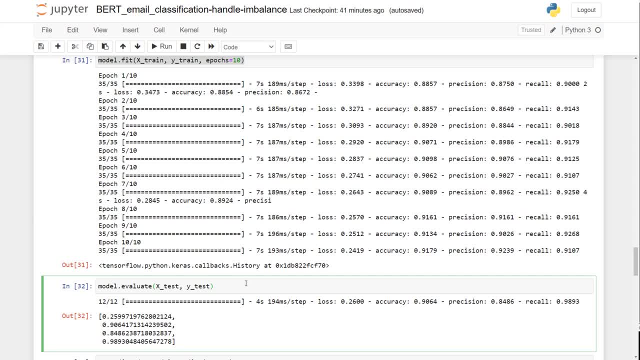 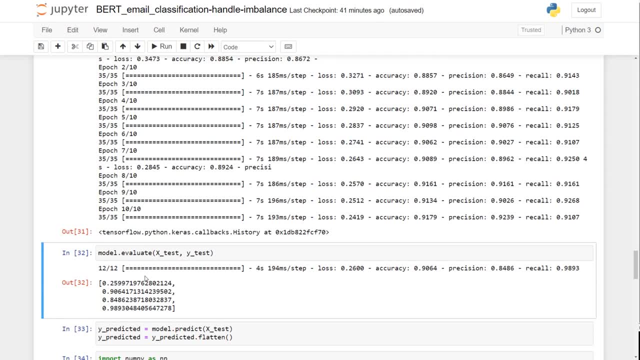 not rely on accuracy- okay, and you can watch my other video. but when you do model evaluation, again accuracy is coming to be 90 percent, which is okay, and then I called model dot predict. and when you do model dot predict, you get your y predicted and y predicted is a two dimensional 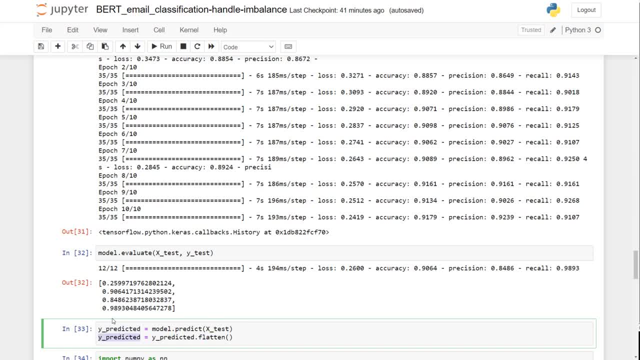 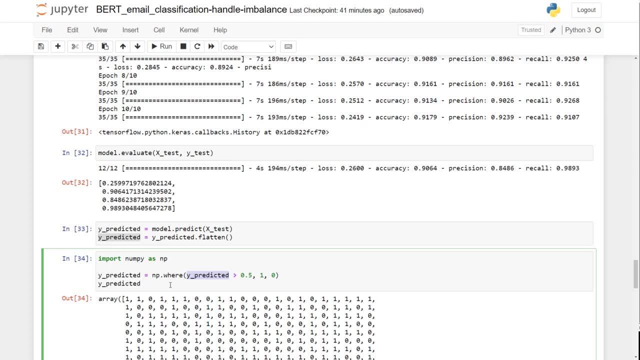 array, but if you do flatten it will become one dimensional array. okay, and then what I'm doing is, since y predicted is a bunch of sigmoid values- point five, point seven, point eight, point eight- what I'm saying is, if the value is greater than point five, put value one. otherwise put value. 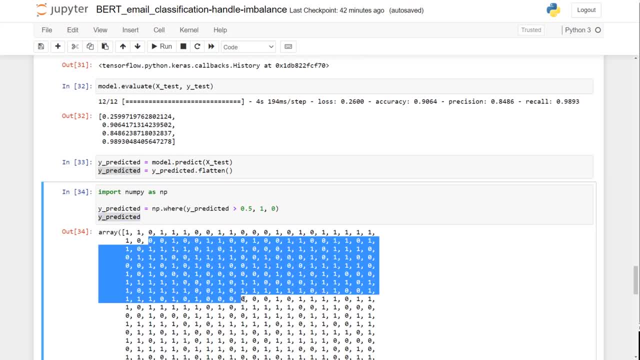 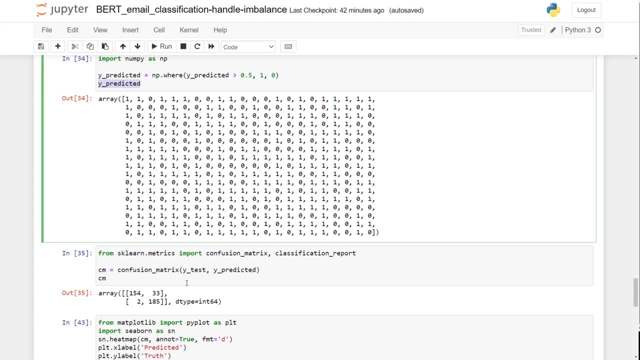 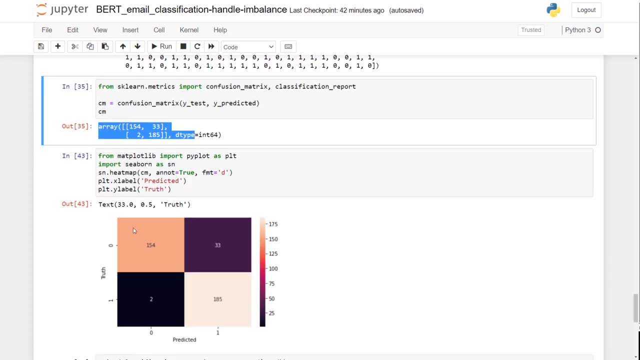 zero. and when I do that my y predicted is a bunch of ones and zeros and then I have my y test. so using y predicted and y test I can plot a confusion matrix here. so this is the same matrix, but I plotted that in seaborn so that it looks visually more appealing. so here what this confusion metric. 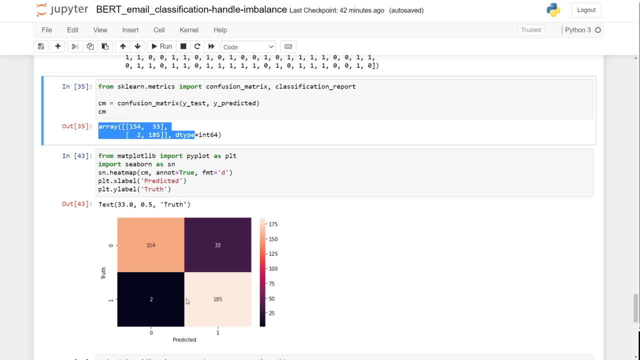 tells you is that on the diagonal, you have your correct predictions. so this is truth. on x, on y axis: x axis is predicted 154 times. I had zero as a truth and my model predicted that to be zero 185 times my. I had a spam email and my model predicted it to be a spam email. 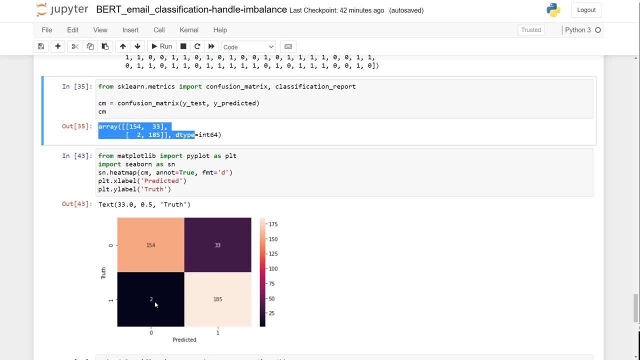 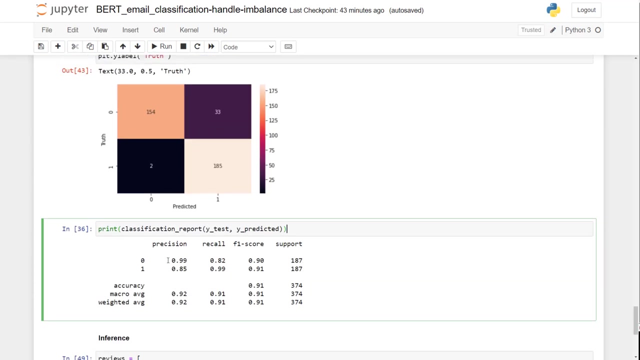 and these are the errors. so on two occasion what happened was I had a spam email but my model says it is not spam, and 33 times the truth. basically, my email was not spam, but it said it is spam. all right when a print classification report, I see good accuracy, good precision and good recall, so it's important that. 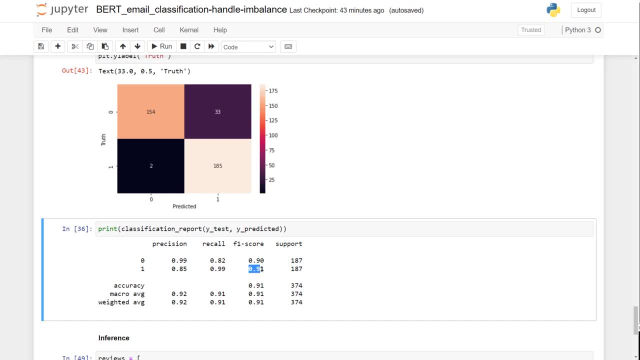 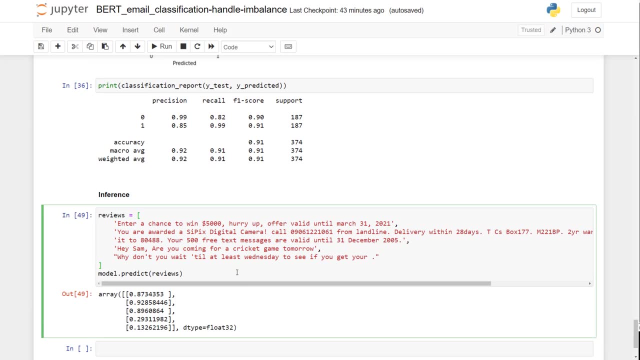 your F1 score is higher. so here, in both the cases, the F1 score came out to be 90 percent and when I do inference on couple of sentences, so see the first three look spammy and the values are: see: more than point five. more than point five means it's spam. 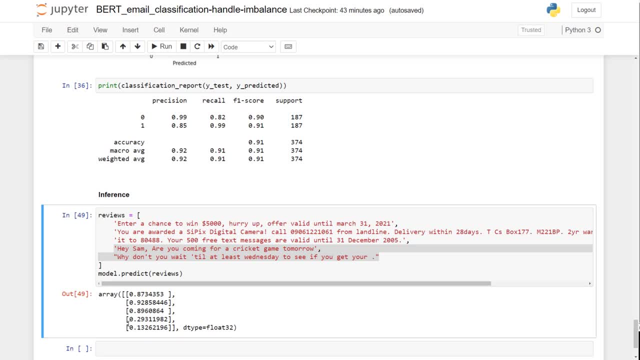 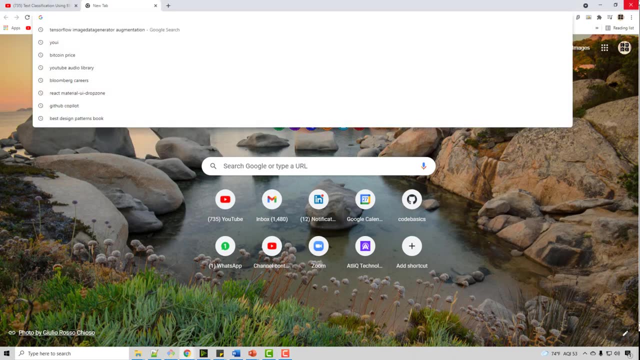 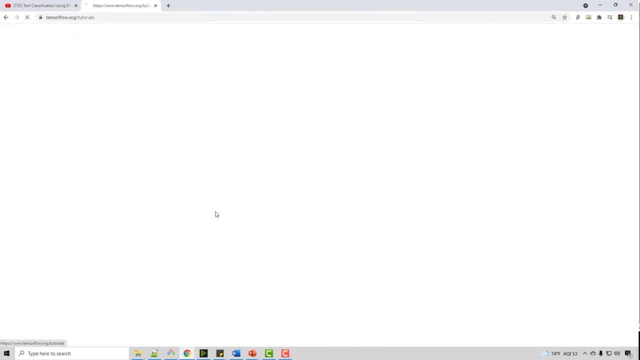 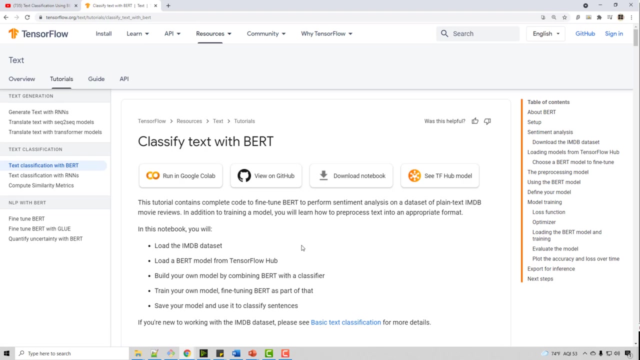 and for these two they are look. they look like legit emails, so the value is less than 0.5. that's all I had for main tutorial. as an exercise, go to tensorflow tutorial. just type tensorflow tutorial and here in the text there is a tutorial called classified text with bird. so the exercise is actually rather simple. 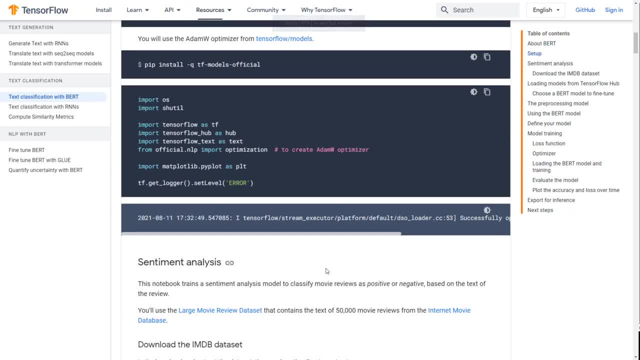 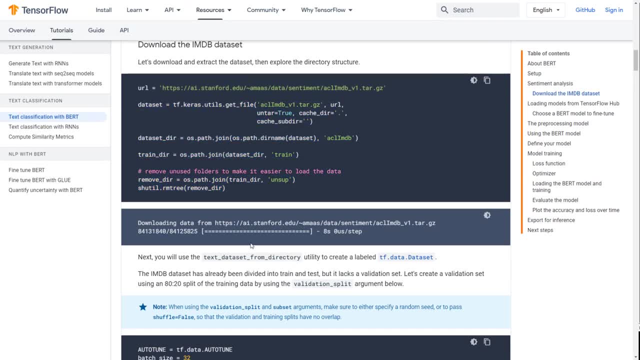 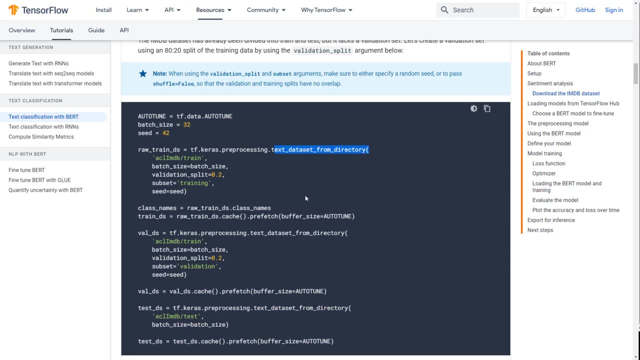 all you need to do is try out this jupyter notebook. it's a ready-made jupyter notebook, but i want you all to try this out. you know, copy paste this code, try to tweak it and try to see how this is working. it is using some advanced aps, text data set from directory, etc. prefetch: we have. 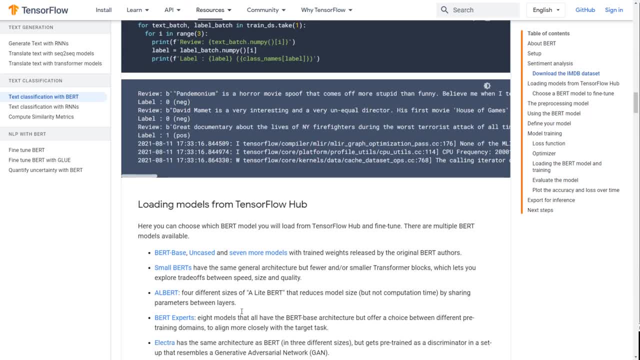 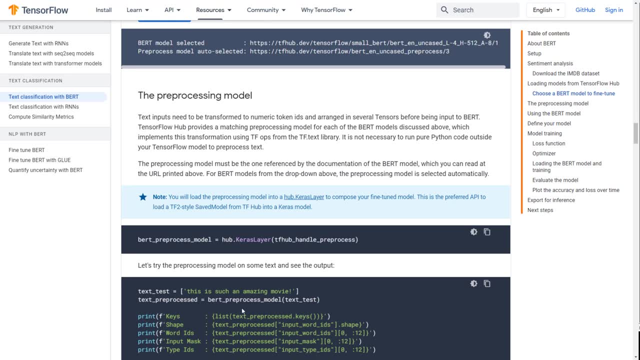 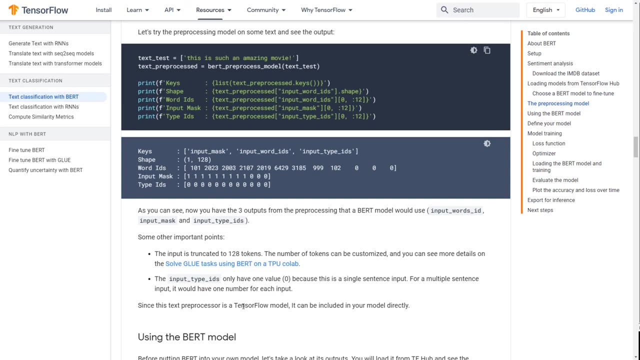 covered all of that tensorflow, data set and all of that, and just try to understand this particular example. it is about movie reviews, but can be used for variety of nlp tasks, such as named entity recognition centers, completion and so on. in our video we just kept things simple. 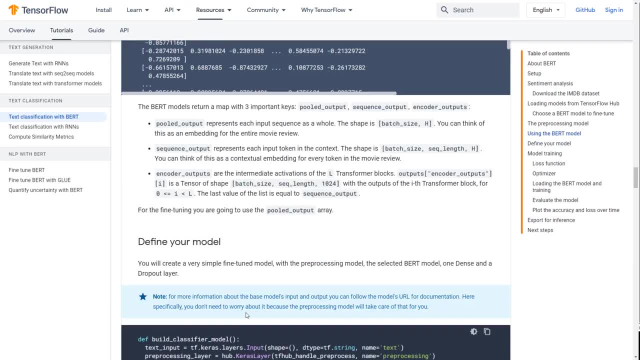 but i i hope you liked it. if you did, please give it a thumbs up and share it with your friends, and please try out this notebook. thank you. 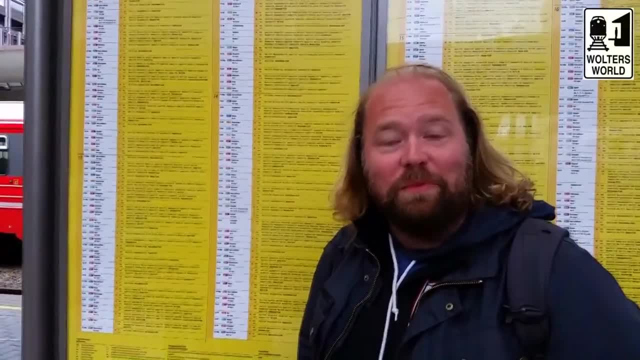 Hi, Mark, here with Walters World, and I got my backpack and we're ready to travel to Gothenburg. And today what we have for you are just some ways that you can tell which train you're supposed to be on, how you can figure out the train timetables here in Europe. So here's. 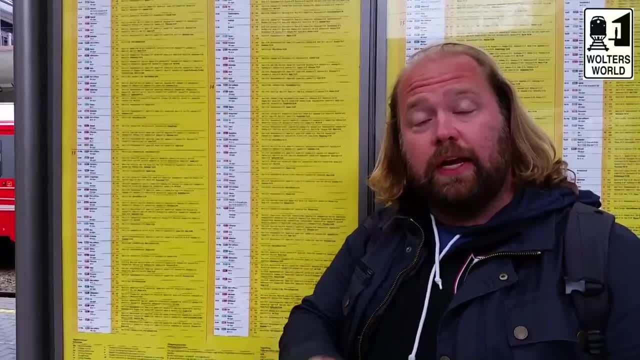 a few tips. The first thing you need to know is the train times in Europe are all on the 24 hour clock, So if it's at 13.30, that means it's at 1.30 in the afternoon. Okay, that's.